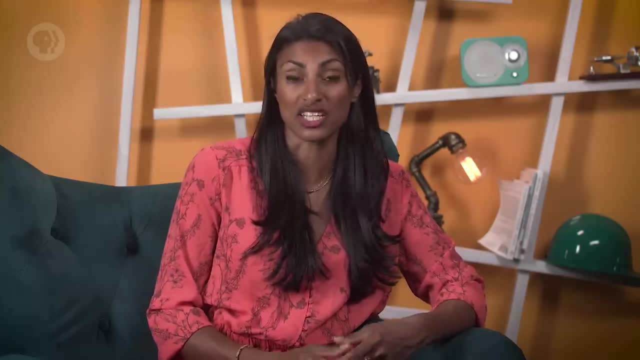 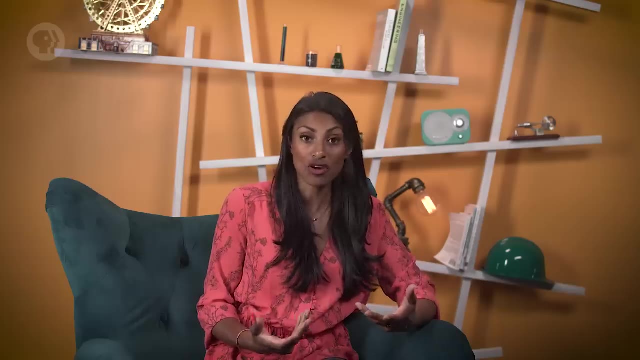 You can then take those bulk materials and form them into stock shapes like sheets, tubes or even powders. That's what you might find at your local hardware or home improvement store. But then to get your final product, you need to turn those stock shapes into a preliminary version of your braces. Even once you have that and make any necessary changes to the design, the braces still need to go through a cleaning process, be checked by quality control and then packaged up before they can be used or sold. That's a lot of steps. 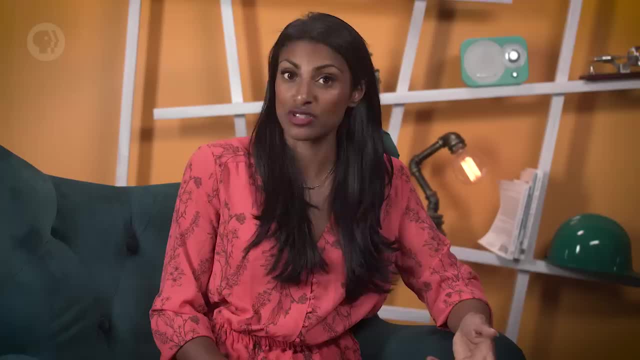 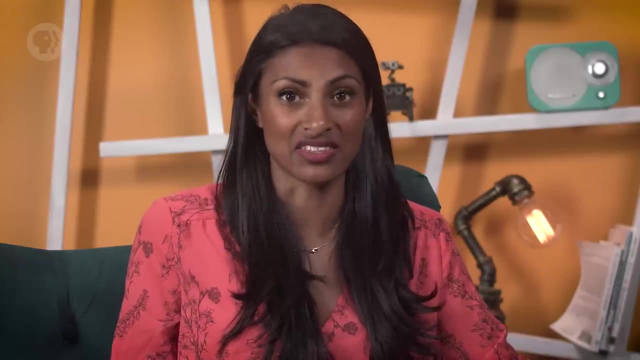 And those are just the basics. In real life there are even more, Not to mention the time and effort it took to pick the right materials, design the brackets and make sure they fit well. You wouldn't want to get all the way to the end and then find out they're just going to snap in half. 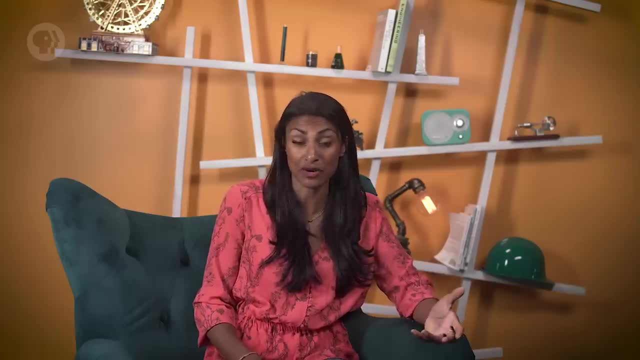 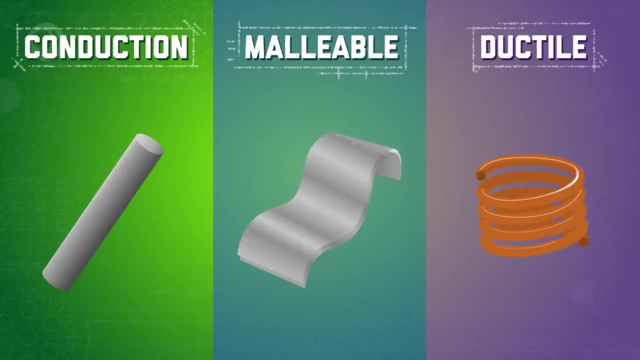 That's why it's so important to understand the properties of the materials you're using. Most metals show a few common properties: They tend to conduct heat and electricity well. many are malleable or easy to shape without breaking, and ductile or easy to stretch and deform. 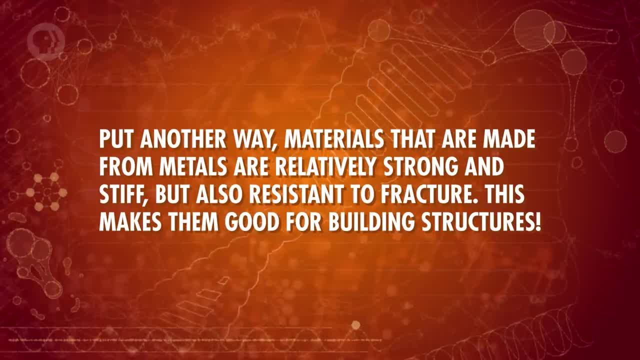 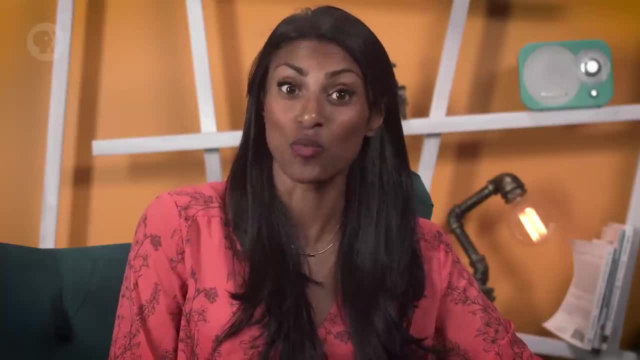 Put another way, materials that are made from metals are relatively simple. Some metals are relatively strong and stiff, but also resistant to fracture. This makes them good for building structures. Metals also typically reflect light well, which is what makes them shiny. That might not be the best if you don't want your braces to be so noticeable. 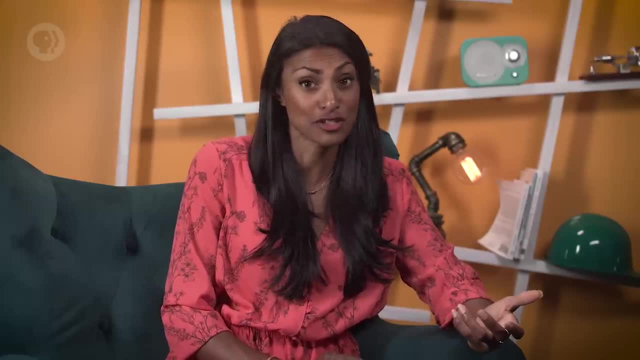 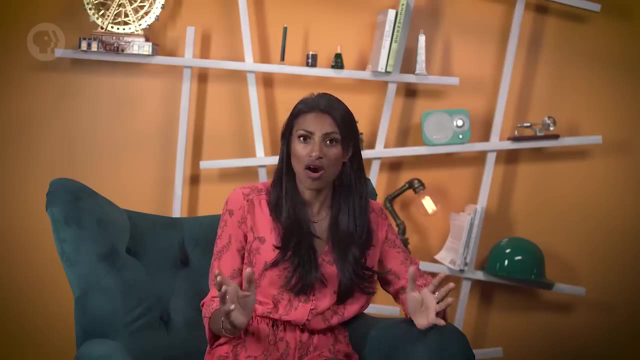 It just depends on what's most important to you – brackets that are less noticeable or ones that are less likely to break. If you decide to use metal in a design for braces or anything else, there are lots of different kinds to choose from. 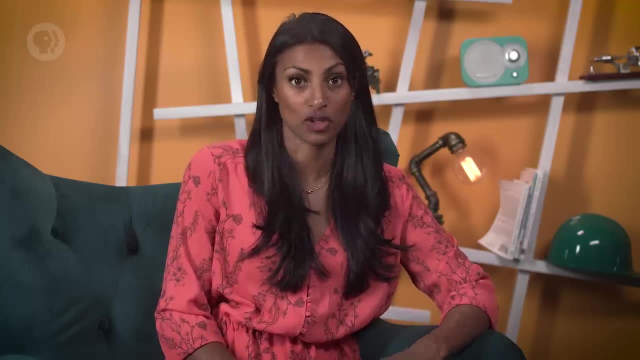 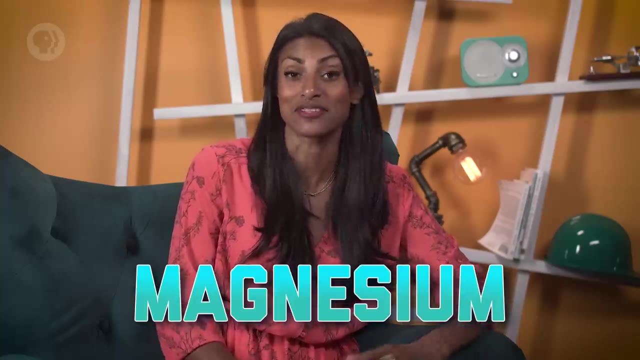 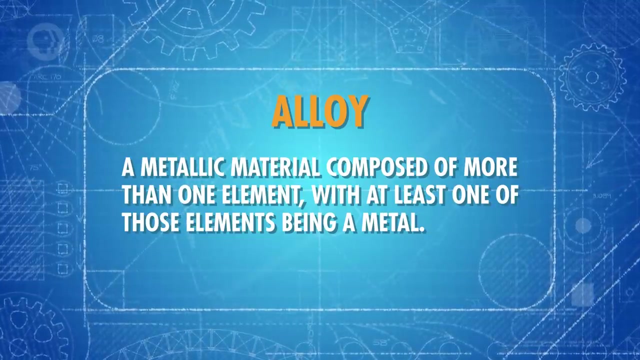 In fact, about three-quarters of all known chemical elements are metals. Common metals that we find here on Earth are aluminum, iron, potassium and magnesium, But often these metals aren't used by themselves. They're added to an alloy – a metallic material composed of more than one element, with at least one of those elements being a metal. 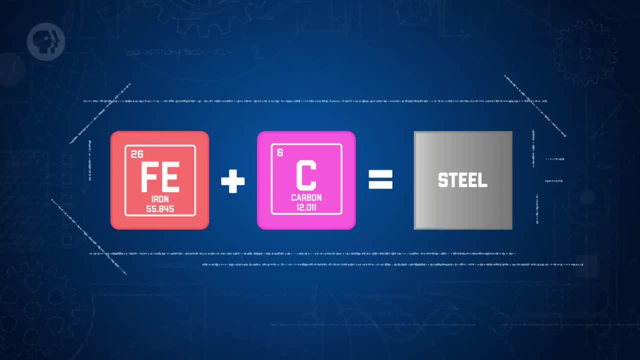 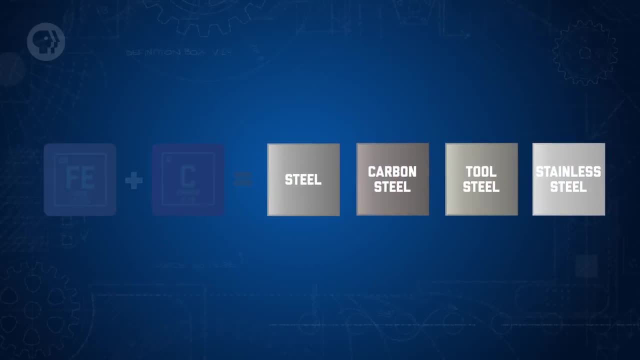 Steel is a good example. It's an iron alloy. It's primarily iron, but it also includes a bit of carbon mixed in. Sometimes there are other elements like chromium or nickel thrown in there too, depending on the type of steel. 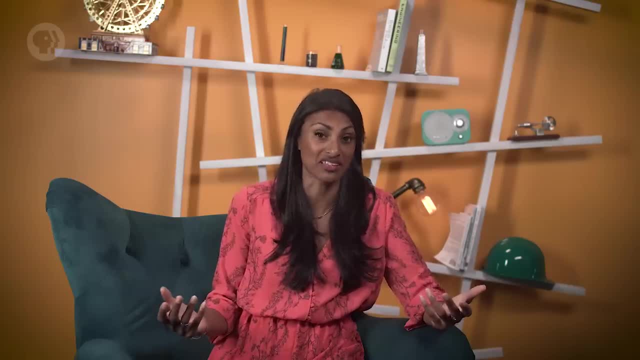 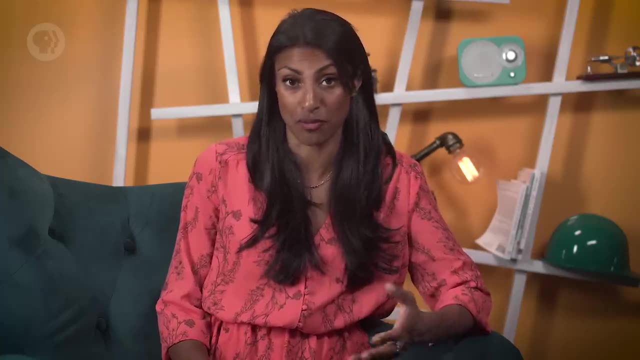 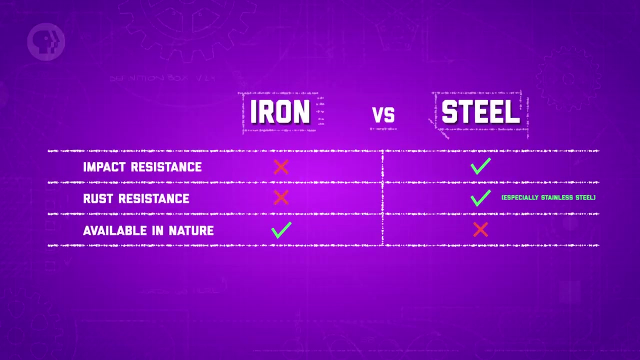 But why not just use the iron itself? Why go through the trouble of making steel, Or any alloy for that matter? It's because alloys have different, and often better properties than the individual elements they're made from. For instance, steel tends to have a better impact resistance than iron, and it's far more resistant to rust and corrosion, especially stainless steel. 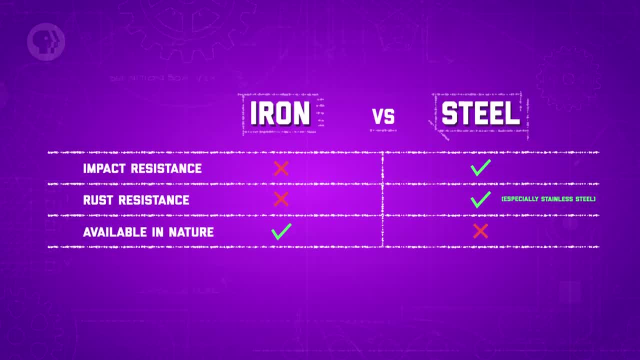 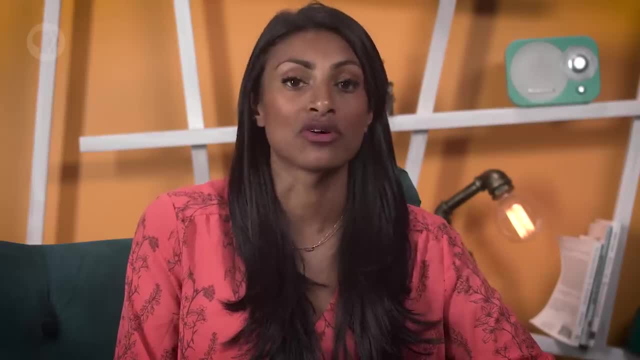 So you'd want to choose stainless steel over iron for projects where corrosion would be a problem, like the exhaust pipe in a car or a replacement joint like an artificial hip. A big reason that metals and alloys are the way they are is because their chemical structure is different. 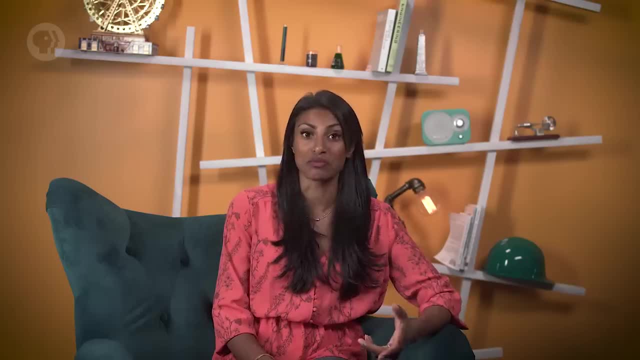 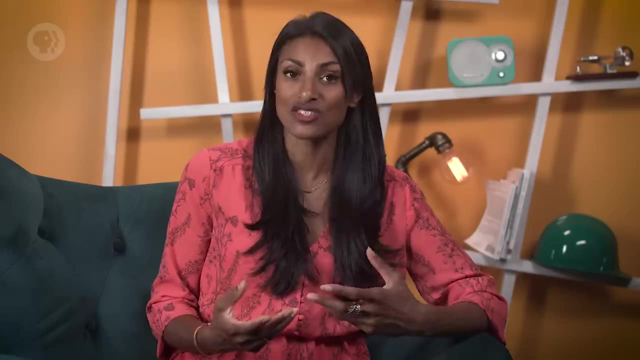 Their chemical structure is more… free-spirited. The bonds within metals and metallic materials leave a large number of electrons that aren't bound to particular atoms and can move from one atom to another. That's known as the free electron theory of metals. 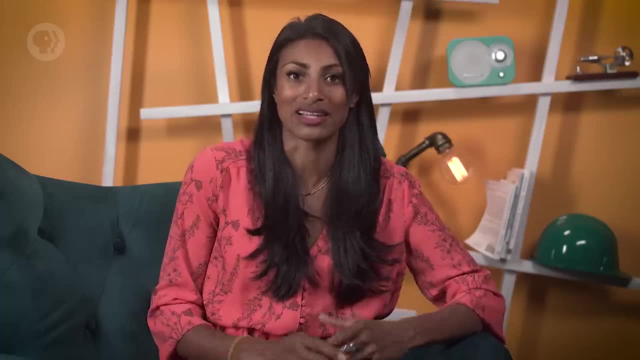 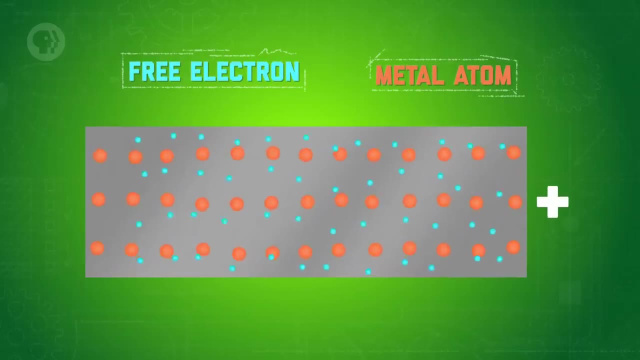 It's like these free electrons can move as a group through the metal itself. This explains why some metallic materials are so good at conducting heat and electricity, Especially simpler metals. their electrons can more easily carry their energy from one place in the metal to the other. 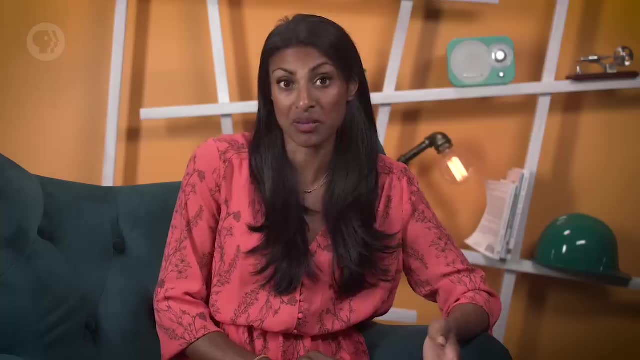 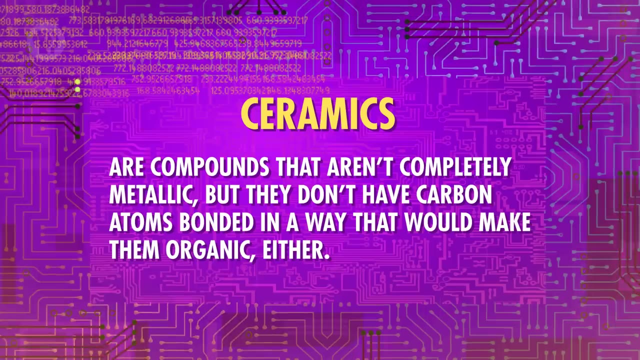 They have positive positives, but they definitely aren't right for everything, which is where something like ceramic might come in. Ceramics are compounds that aren't completely metallic, but they don't have carbon atoms bonded in a way that would make them organic either. 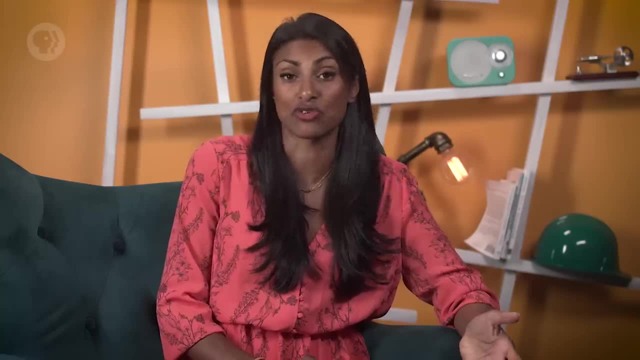 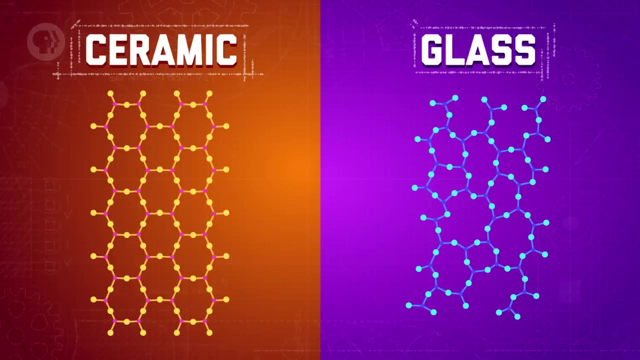 You can define glass materials in the same way, so a lot of people include them in the same general category. The main difference between glass and other ceramics is their chemistry. Ceramics are usually crystalline, which means their molecules are more ordered, whereas the molecules in various types of glass are more random. 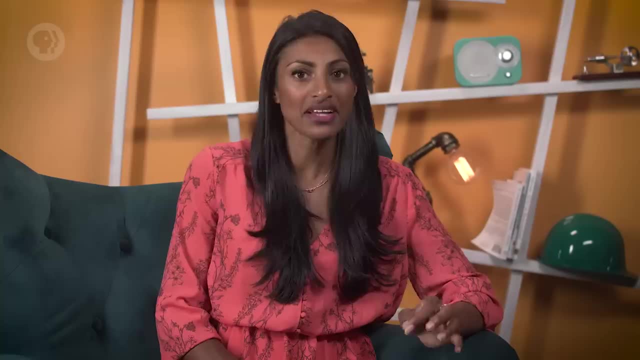 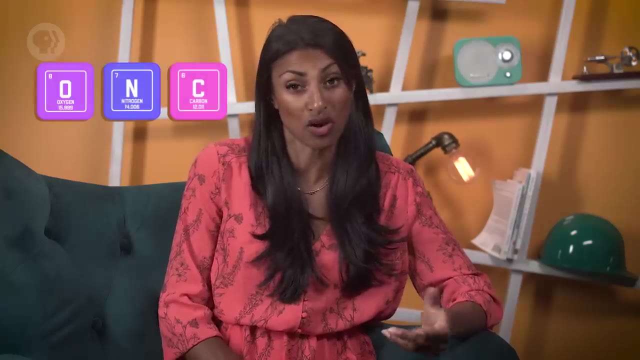 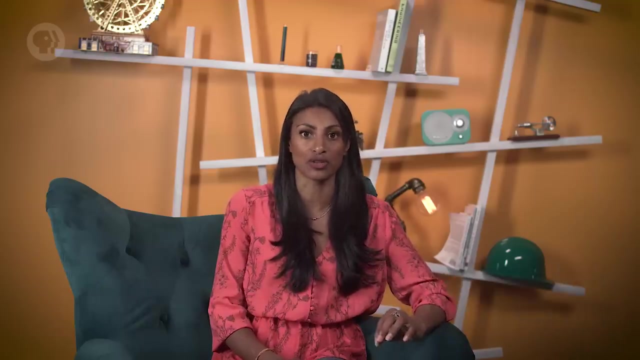 In terms of how they're organized, the molecules in both ceramics and glasses are made up of at least one metallic element plus at least one non-metallic element. They often include oxygen, nitrogen or carbon. Common examples include aluminum oxide, better known as rust, and silicon carbide, which can form a very hard material that's used to make everything from car brakes to bulletproof vests. 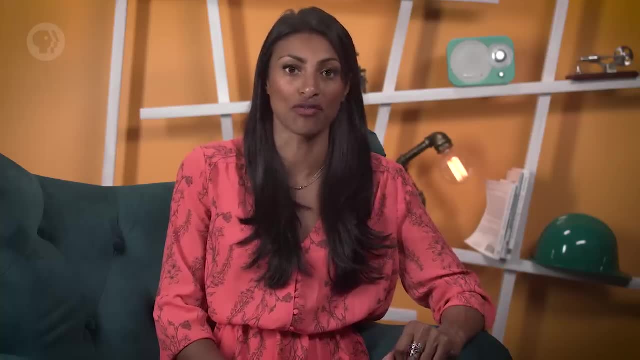 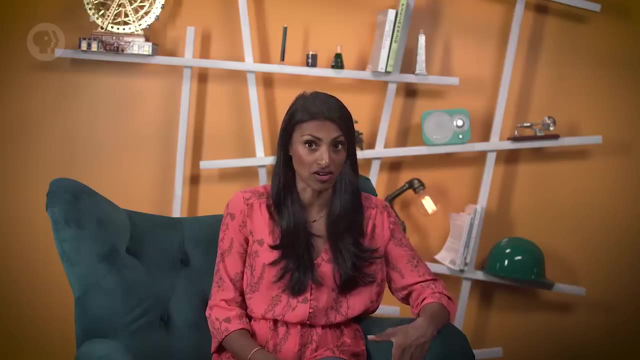 And, of course, there are the more traditional ceramics that most people think of, like cement or compounds made of clay materials like porcelain. In general, ceramics are relatively stiff and sturdy. In this way, they're similar to metals, But they're also extremely brittle and can fracture very easily. 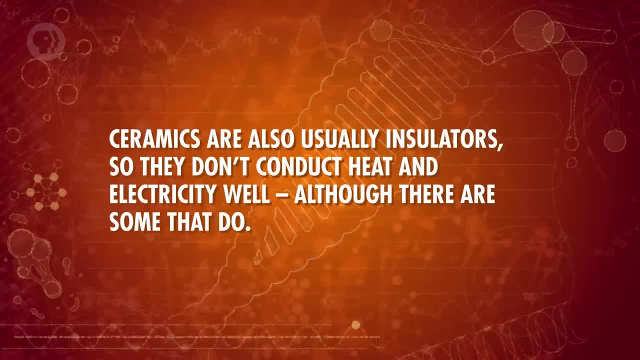 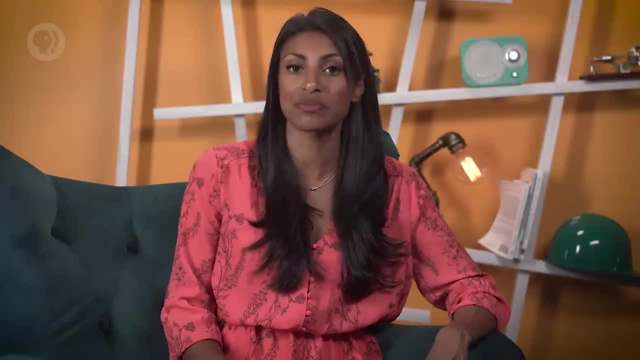 Which doesn't sound too good if you're going to have them on your teeth for a few years. Ceramics are usually insulators, so they don't conduct heat and electricity well, although there are some that do, And they tend to be more resistant to extreme temperatures and harsh environments than metals and polymers are. 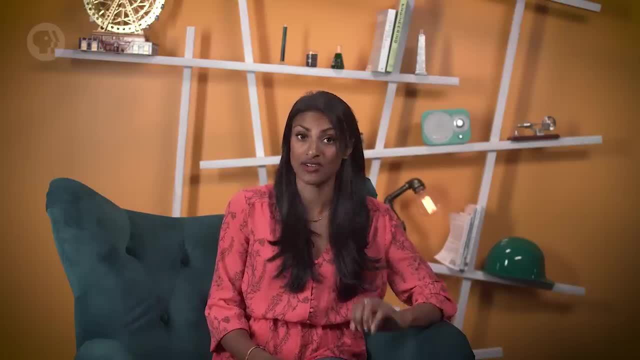 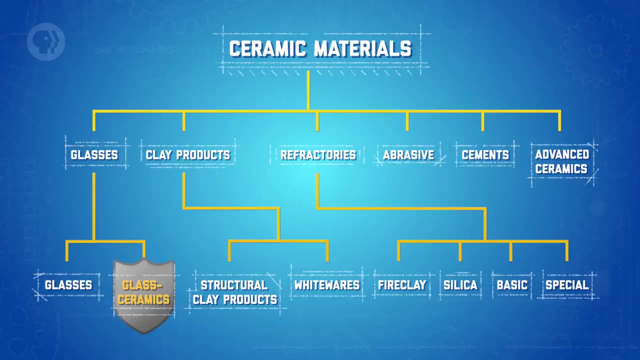 But while most ceramic materials have similar properties, there are differences. We could spend hours going through all the different types of ceramics out there, but there are a few major ones: Glass Ceramic Materials, Glass ceramic materials or materials whose chemistry falls between glass and other ceramics are relatively strong and don't melt easily when heated. 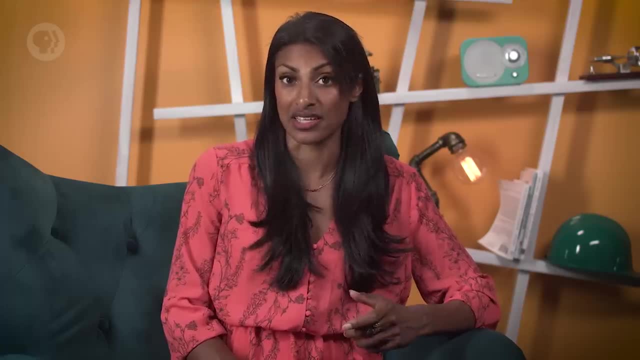 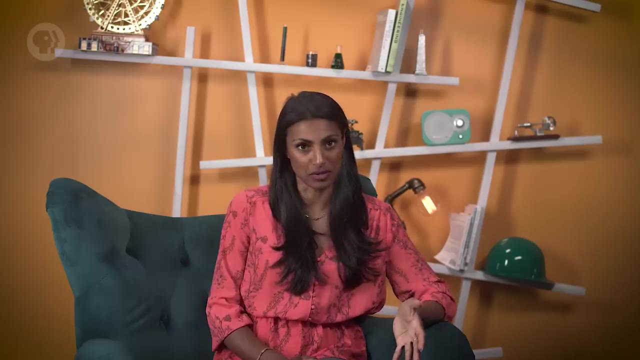 They also tend to be biologically compatible and they make good insulators, which is why they're commonly used in electronic packaging applications. Plus, they can be completely transparent. Perhaps one of the biggest appeals of glass ceramic materials is how easily you can fabricate them. 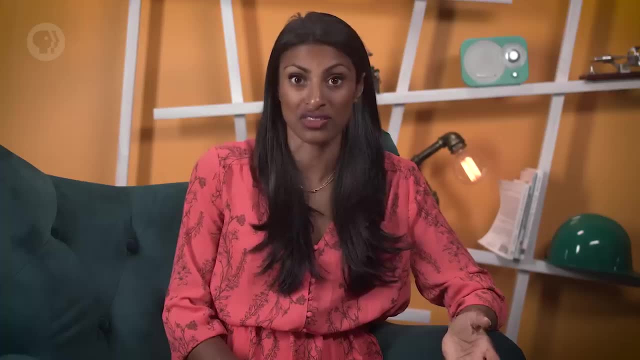 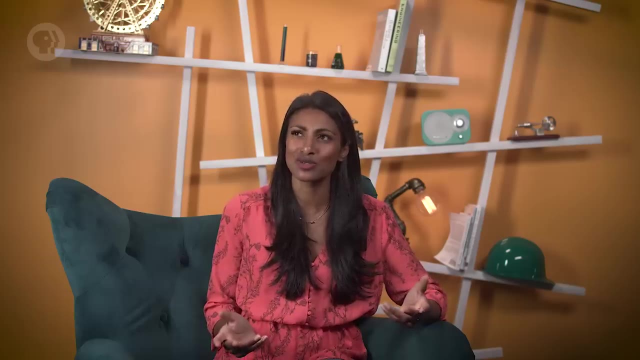 You can use conventional glass forming techniques and you end up with a product that's nearly pore-free, which is great for handling liquids. So glass ceramics are really useful. Sometimes you want something a little… simpler, like clay. Clay is inexpensive and commonly found in nature. 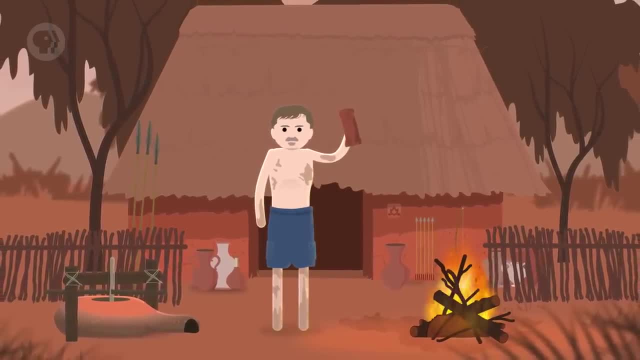 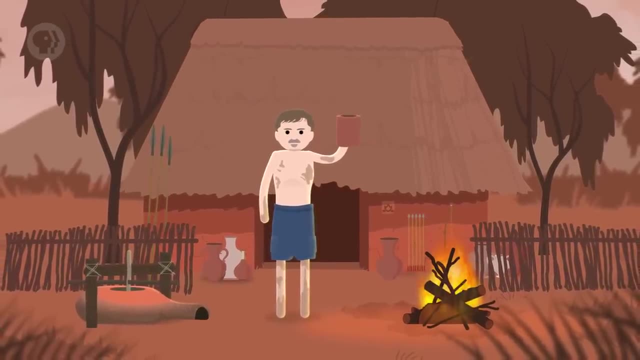 You can often use it as-is after mining it, meaning that you don't need to waste time or resources on refinement, and it's super easy to work with. If you've ever taken a pottery class, you know that clay and water, when mixed in the proper proportions, forms a material that's easy to shape. 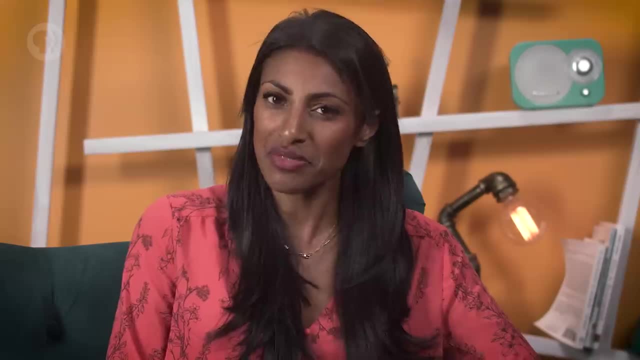 Put that through a kiln and you've got something great for mugs and dishes. For something a little sturdier, you might try using cement. It's mainly used as a binder to help hold concrete together, which means you can find it anywhere. 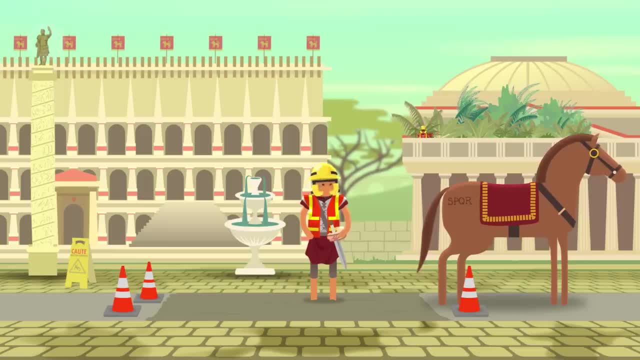 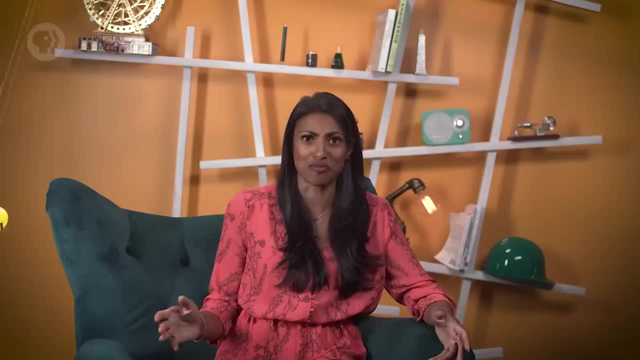 From roads, dams and buildings to more decorative applications like patios and staircases. One big benefit of using cement is that it can set at room temperature. Imagine if you had to break out some big flamethrower every time you wanted to pave a new road. 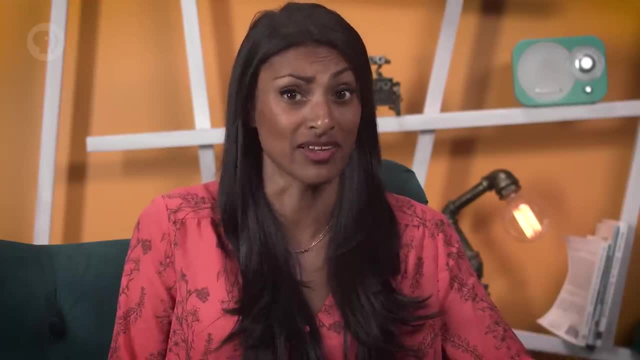 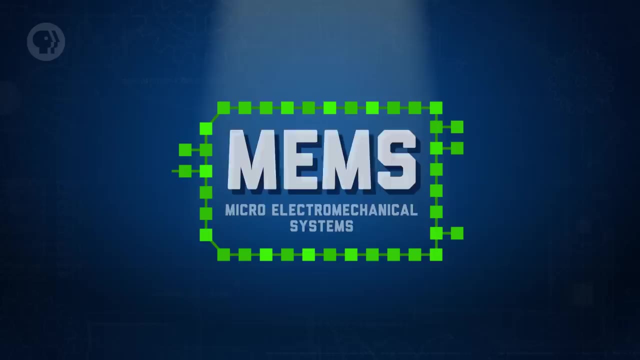 So yeah, you could say cement's properties make it an important part of our lives. Ceramics and metals also show up in places you might not expect them, like with microelectromechanical systems or MEMS. These are miniature smart systems that use tiny sensors to collect information by measuring things like mechanical energy. 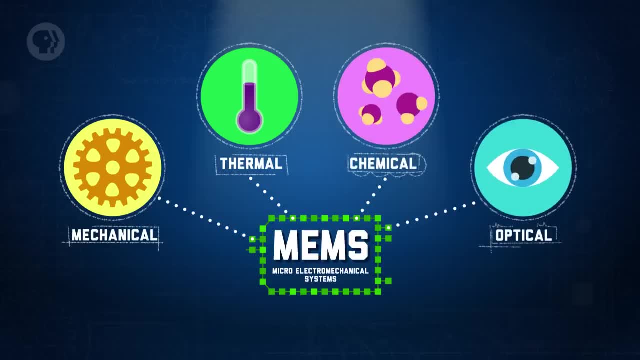 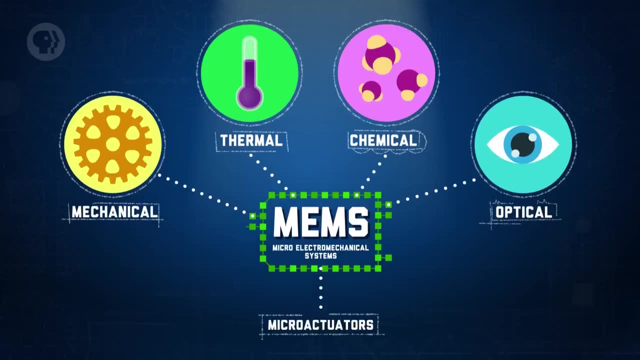 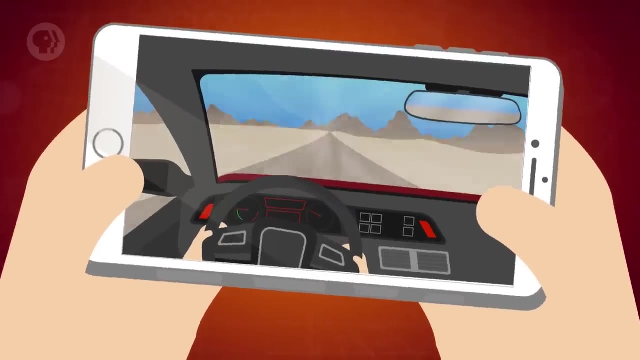 They use the information to make decisions that tell devices called microactuators to do something like move a fluid or redirect a beam of light. A major application of MEMS these days is something you probably know pretty well – the accelerometer, For example. there's one in your phone to detect its movement, and cars have accelerometers that trigger the deployment of airbags during a crash. Compared to older and more conventional airbag systems, ones that use MEMS are smaller, lighter and more reliable and quite easy to use. So what's the difference? They're more reliable and quite a bit cheaper to produce, And with something as important and life-saving as an airbag, those are big benefits.